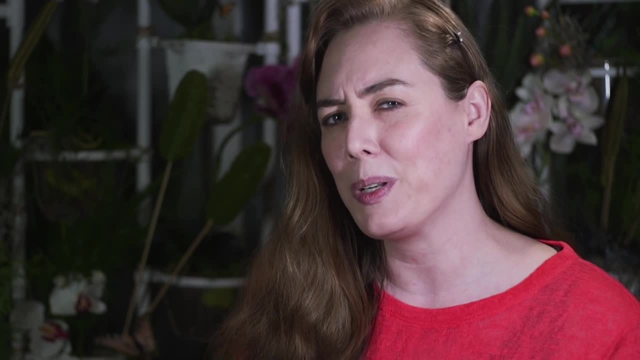 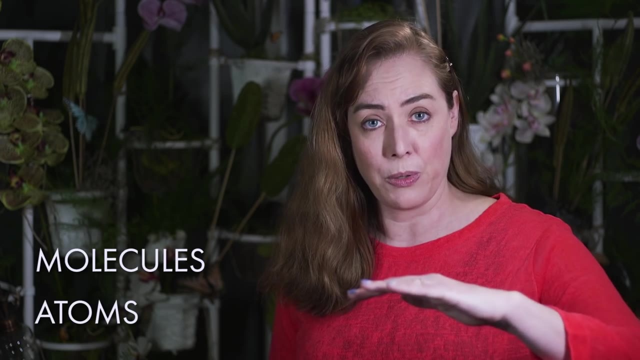 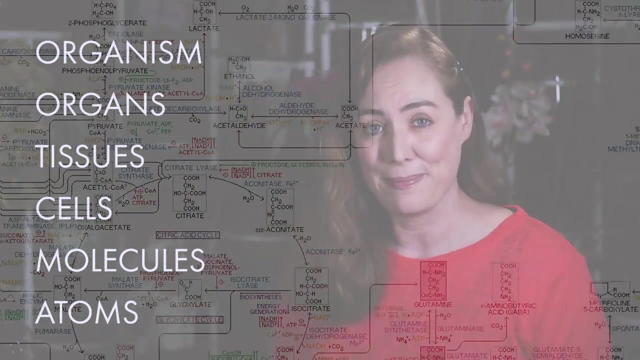 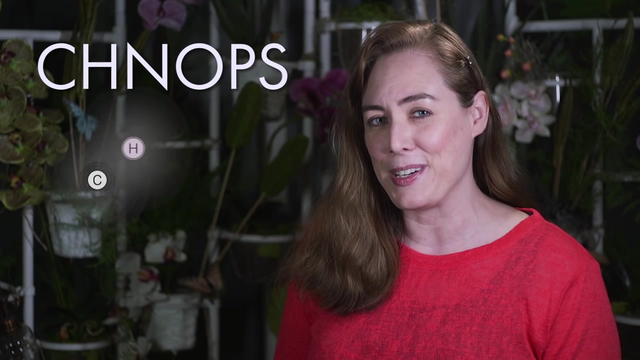 and interact, properties emerge that you wouldn't predict. You can think of biology in terms of a structural hierarchy — atoms, molecules, cells, tissues, organs. Pretty soon you have a multicellular organism with a metabolism. Let's start with atoms, especially schnapps — carbon, hydrogen, nitrogen, oxygen. 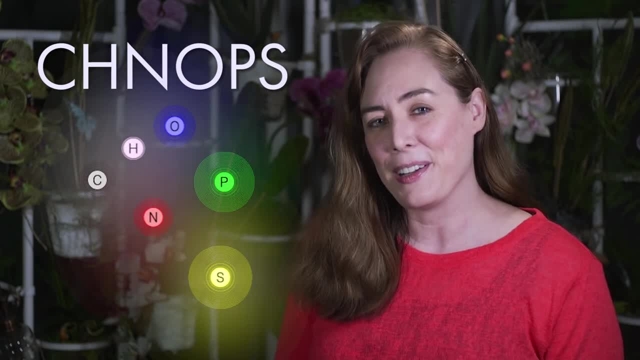 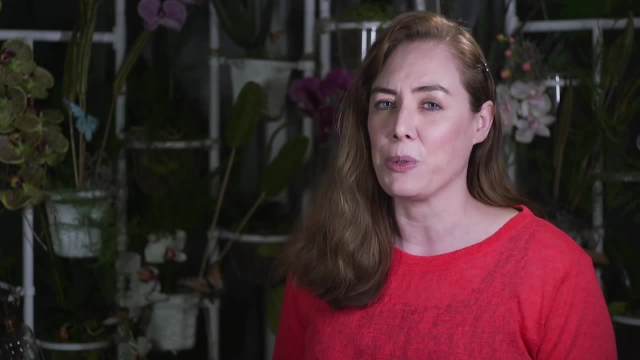 phosphorus and sulfur. These are the elements that make up a cell's body and the cell itself. You can buy a cell from any company you like — make up 98% of living matter on Earth. We can study the behavior of these individual atoms. 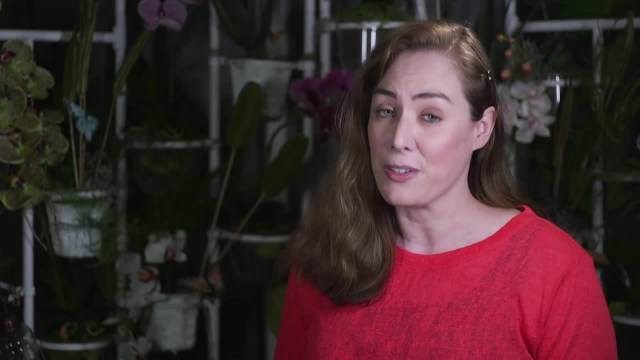 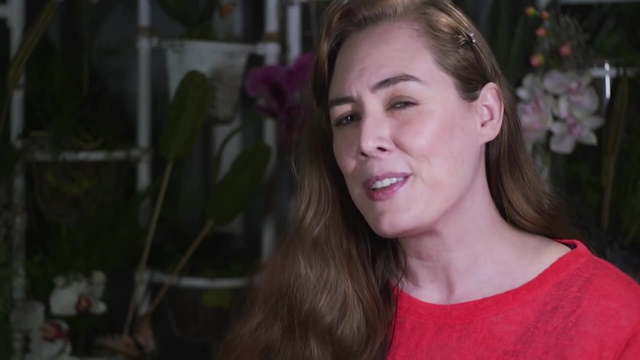 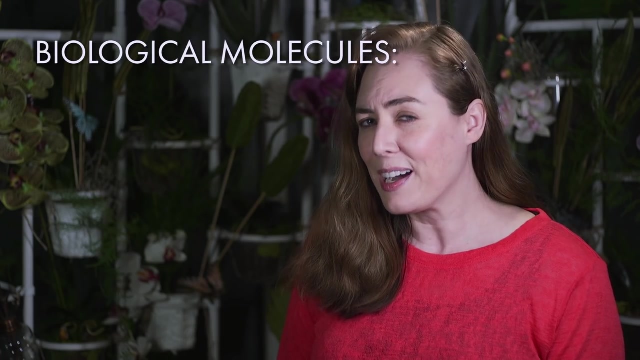 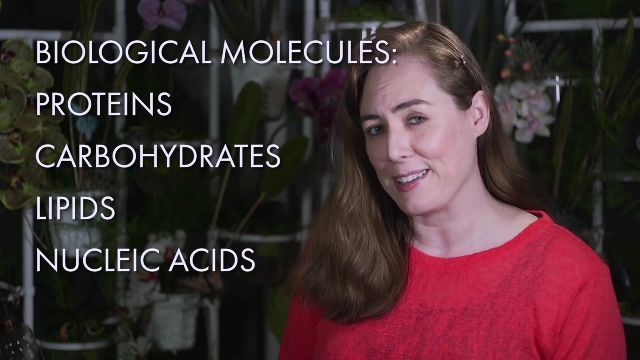 but things get more interesting when these atoms interact. Bonds are formed and broken. We see the emergence of chemical behavior. Some of these atoms stay bonded together, forming biological molecules. There are four main kinds of biological molecules: Proteins, carbohydrates, lipids and nucleic acids. Proteins are polymers of amino acids. 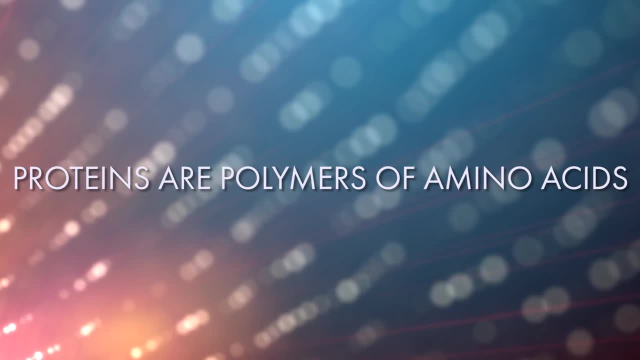 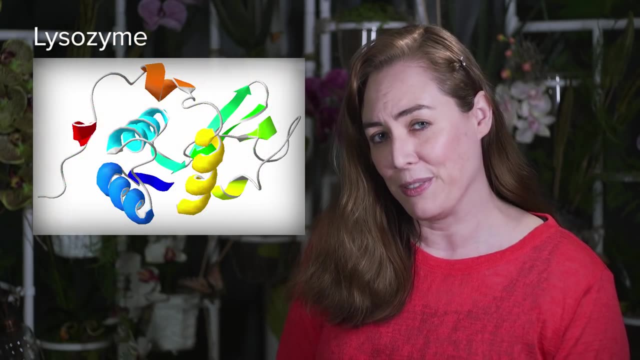 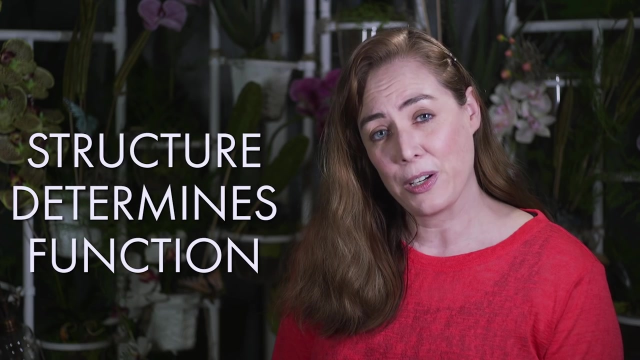 That is, amino acids strung together to form a chain. These strings of amino acids fold into three-dimensional shapes that do most of the work of life With proteins and all biological molecules. the key to remember is that the 3D structure determines the function. 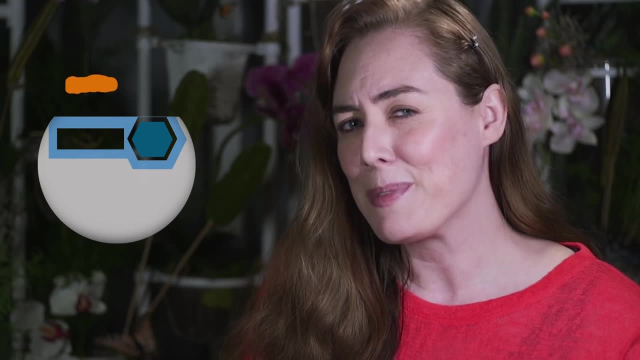 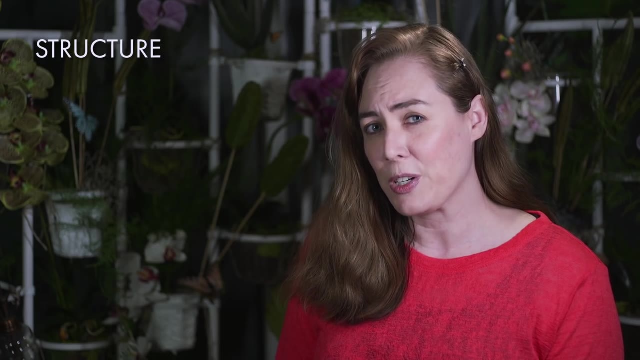 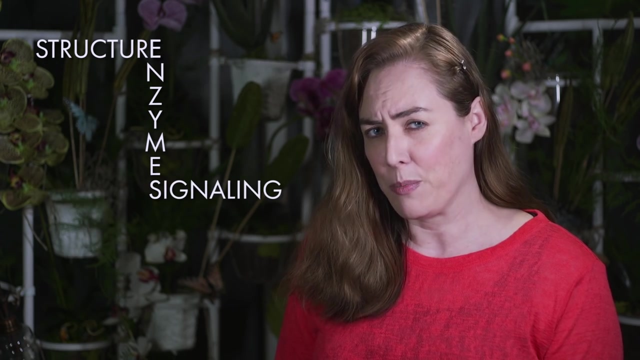 Think of how a key fits into a lock. The shapes have to be just right for the key and the lock to do their jobs. The jobs of proteins include structure like collagen, Enzyme catalysts that control the rate of reactions, Signaling, like some hormones, Immune function like antibodies. 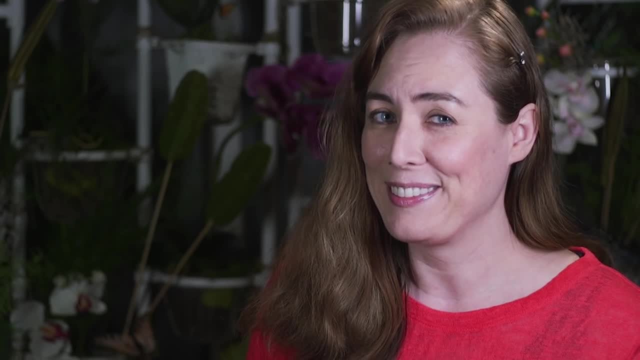 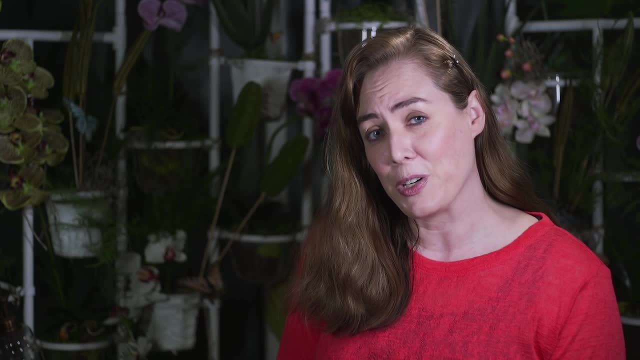 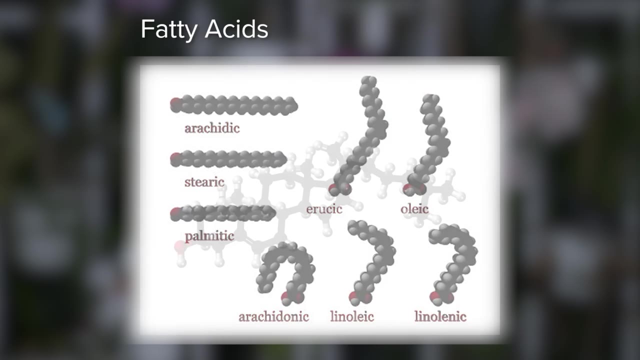 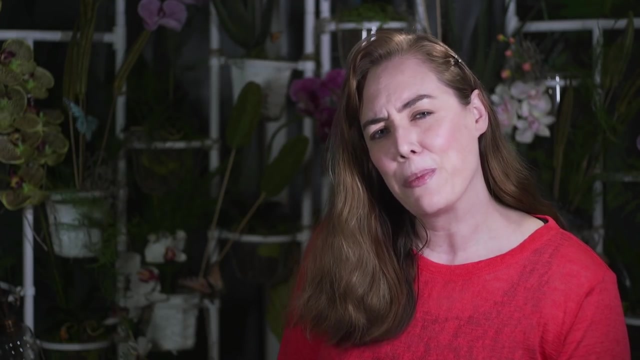 carbohydrates are sugars and polymers of sugars. These are used for energy and to build biological structures. Lipids are non-polar molecules like fats, oils and phospholipids. These are important for energy storage, for cushioning and for structures like cell membranes. 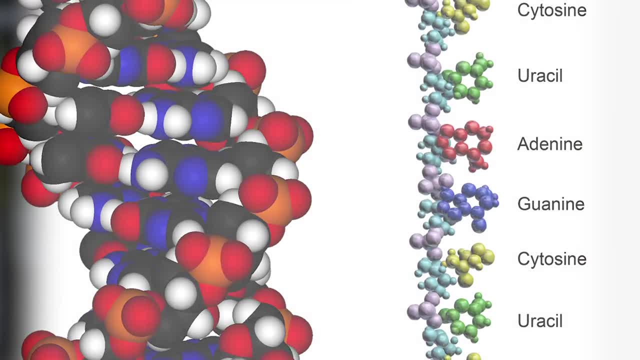 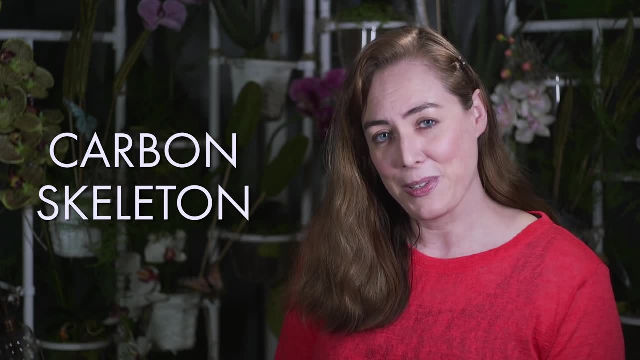 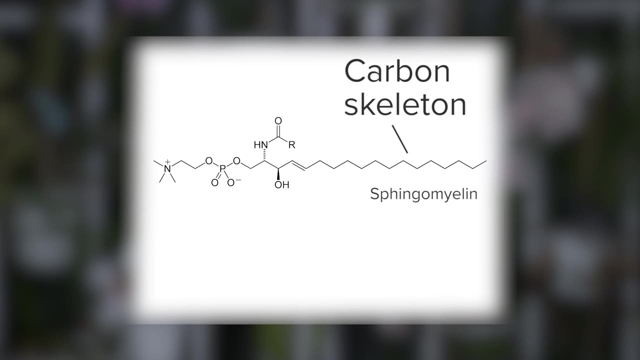 Nucleic acids include DNA and RNA. These store genetic information. It's important to note that these are all carbon-based molecules. this is why we say we're carbon-based lifeforms. The skeletons of biological molecules are made up of carbon atoms covalently bonded together in very stable structures. 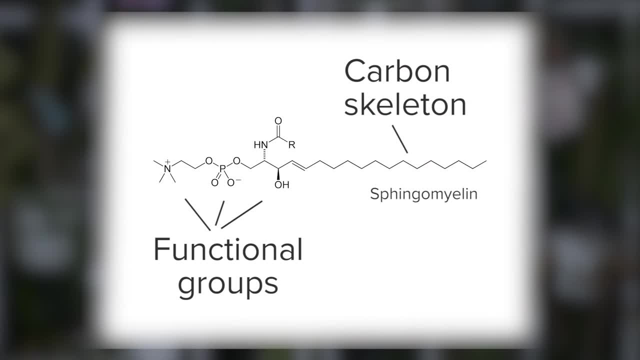 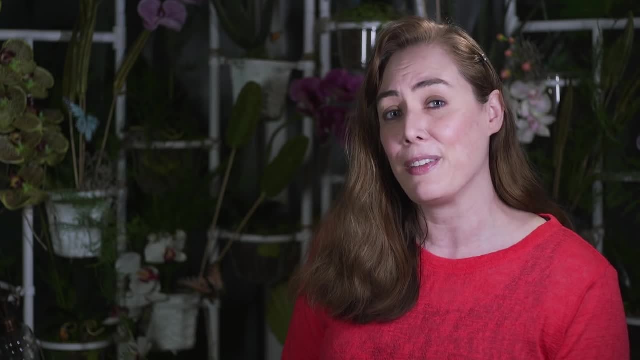 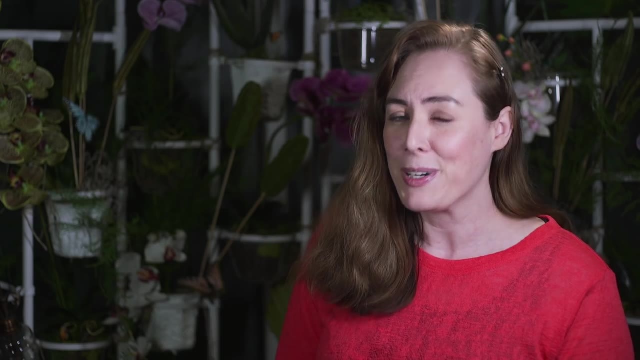 Hanging off the outside of the molecules are functional groups, small chemical species like OH or CH3. Think of the carbon skeleton giving biological molecules their general 3D shape- and the functional groups like flora and fauna are functional groups. We don't have to fuss. We have those flags hanging off. participating in chemical reactions. 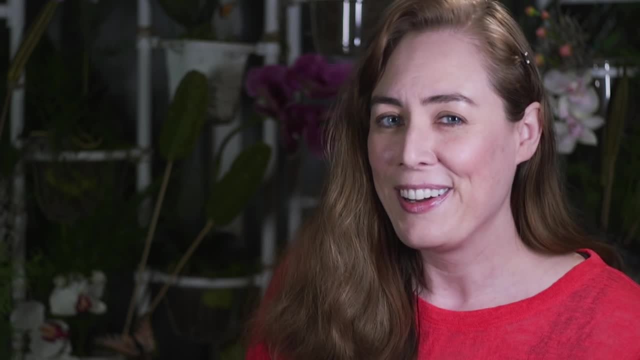 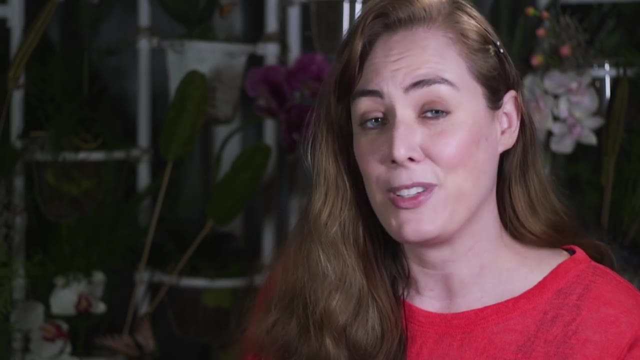 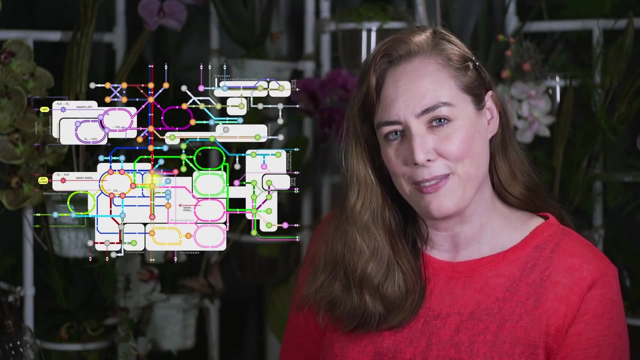 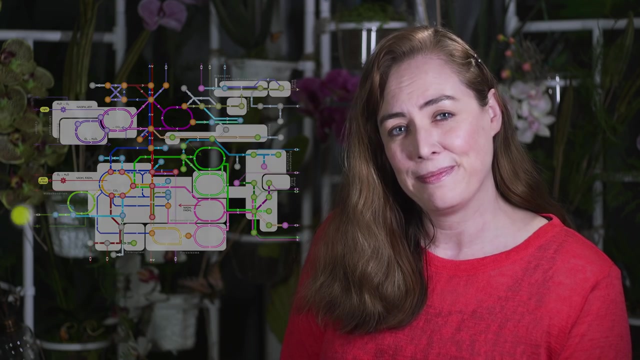 We see another level of complexity emerge when these biological molecules interact with each other. We get enzymes controlling reaction rates, We get DNA replication genetics, We get cells… And… within cells, we have an incredibly diverse set of chemical reactions that are the right rates to keep us all alive. That's what biochemistry is: The building blocks of life itself. 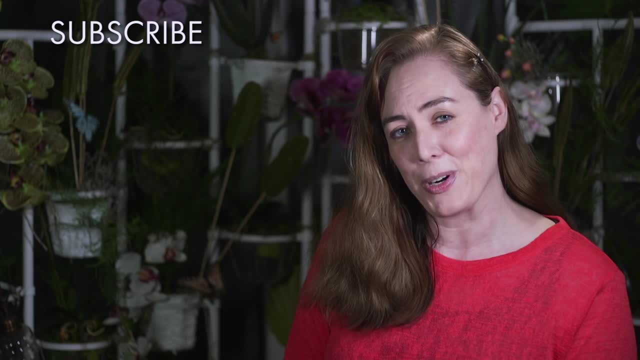 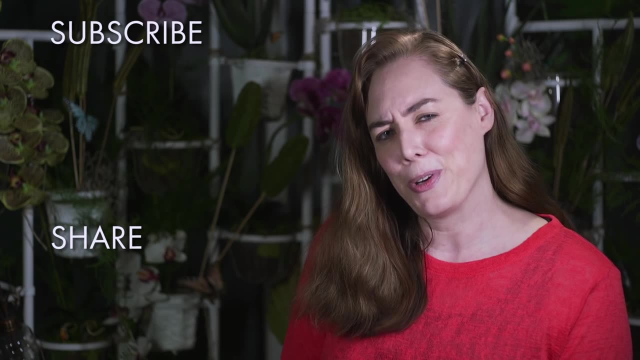 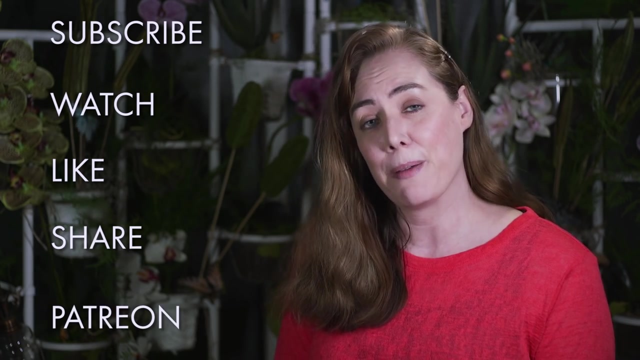 Our new biology series will cover all of these topics in more depth, so be sure to subscribe so you'll find out when we release each video And share these videos with your friends. They need to learn all about biology too. If you'd like to help us make more videos, you can become our patron. 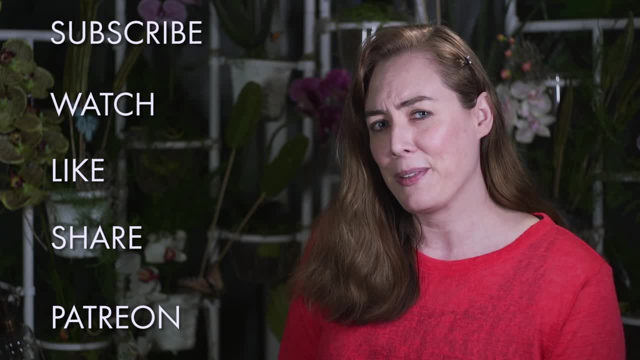 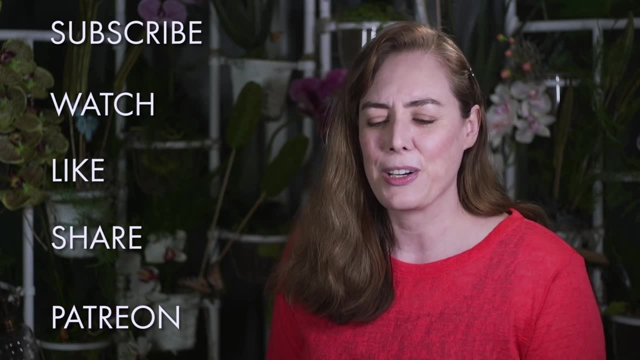 on Patreon. If everybody donated a dollar a month, we'd be able to have a crew of professionals instead of just me in my greenhouse. Like share, subscribe, Patreon. Did I leave anything out? You can let me know in the comments. 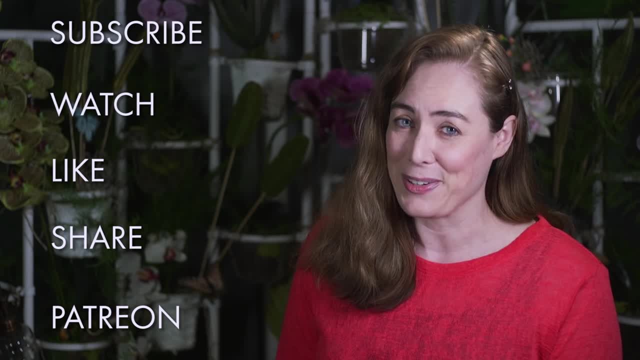 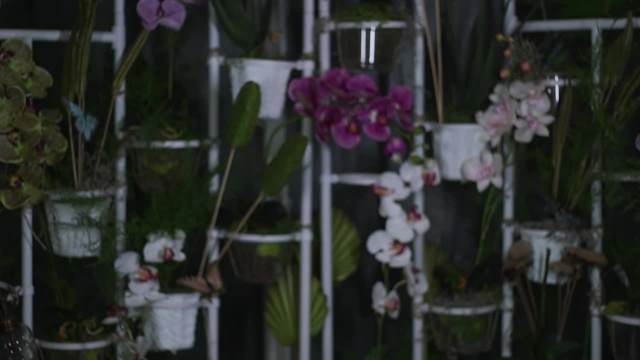 And be polite. We expect you to keep it clean here at Socratica. Thanks for watching. I'll see you in the next video.